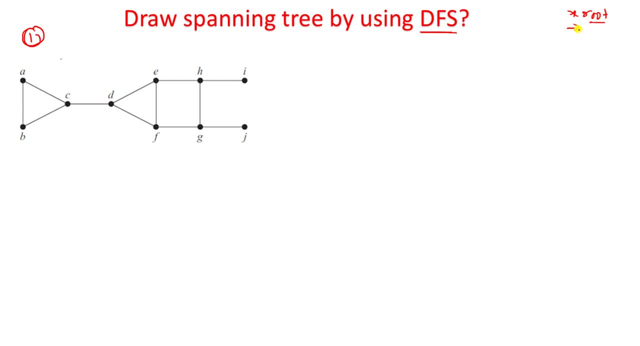 Okay, not all the vertices, not all the incident vertices. we have to choose only one vertex, that is DFS. So here, what is our root node? A is our root node, right? Okay, good, Now write down here. this is a rough work, Ma, No need to write in the exam. Okay for your. for a better understanding, I write here like this For A: how many incident vertices? A have the edge with C and B? right, So then can we take all the C B? No, just we have to explore. 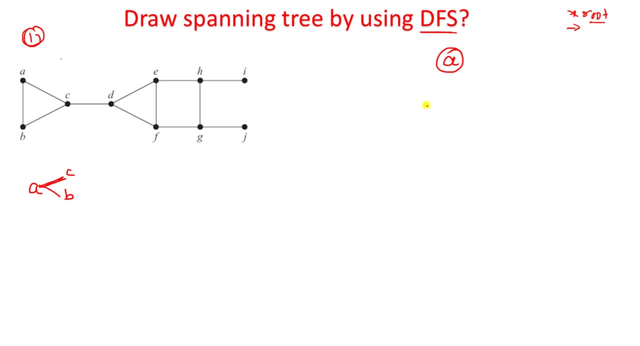 explore only one vertex. we have to explore only one vertex called what c. okay, so i take c as a next vertex. and next where, where i am, i are in c. okay, i am at c. now explore this c. uh, what are the vertices? it incident with c, so c have a and b and what d? okay, so here you can take any one of them. 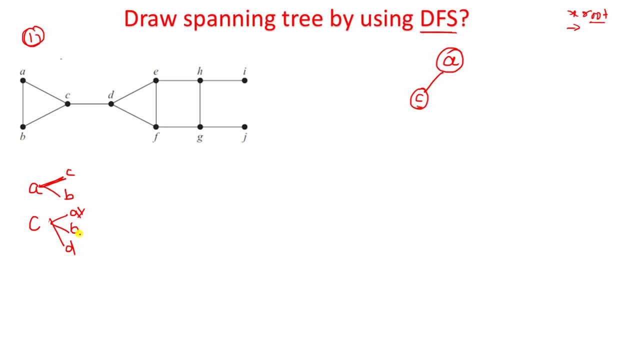 but a, you will already visited, so you can eliminate this one. and next one: b and d. so among b and d, you can take any one. b or d, okay, but i choose d here, i choose d, here you can. you can take b, okay, no problem, but here i choose what? uh, d, okay, and then what is the next one? what is the next one? 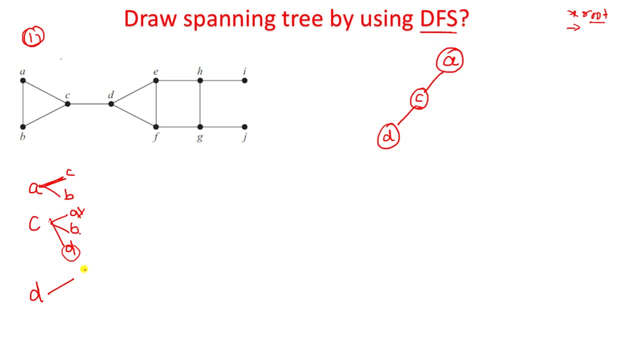 is the next explorer vertex, that is d. so d have a edge with c, and the next e and the next f. okay, and the first, what is the first one? c is the first one, so, uh, it is already visited, so no need to take it again. and the next element is e and f. okay, so i take it as a, e, e as my next vertex. okay now. 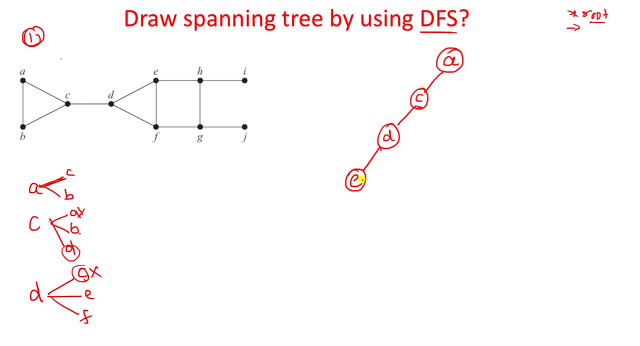 what is my new vertex? e explore this vertex and write down only one vertex incident with the e. so e having connection with d and f and h. right, ma? so d, h, three connections are there. okay, so d already visited. no, so you can uh, eliminate this one and f and h. so among f and h, you can eliminate you. 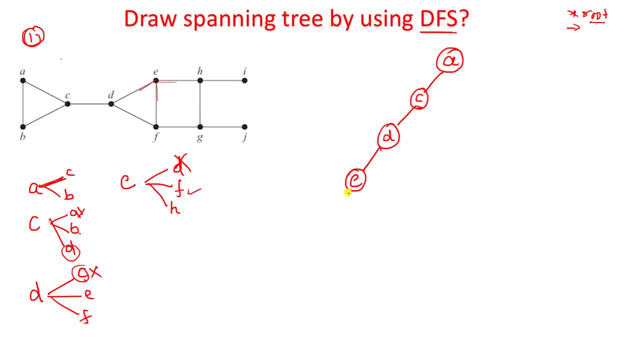 can take any one. so i can take f. okay, f as a next vertex now. what is the next vertex? f. now write down what are the next incident vertex for the f? f have a connection with the d, e and g and e. right, three, three are there: f to d, f to e and f to g. okay, so d is already visited and 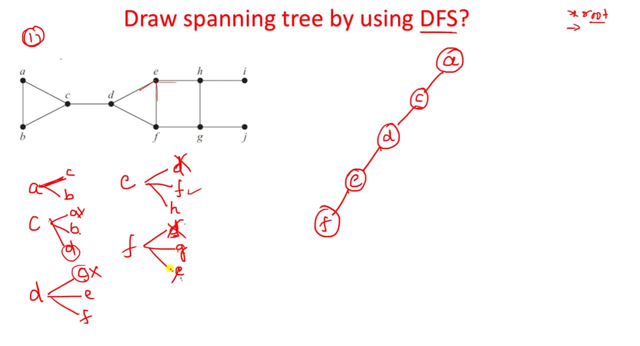 what about g? g is not visited, but e- e already visited. first remove the visited vertices. okay now, first remove the removed waste visited vertices. so only element is what g, okay, fine, now write down what is the next element for the g. for g, we have, uh, how many vertices. f and h and j, okay, so first remove what already visited. 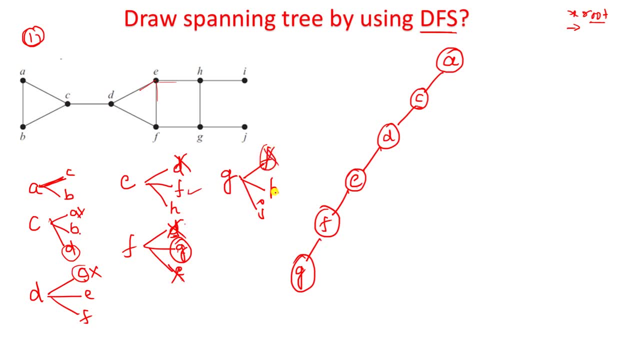 vertices f is already visited and h, h not visited and j, j is also not visited. okay, for g, i can insert: uh, i can take h, okay, i can take h. or you can take j, i can take j, i can take j, i can take j, okay. so here our new vertex is what j, so explore this j, what you will get after visiting, so j having. 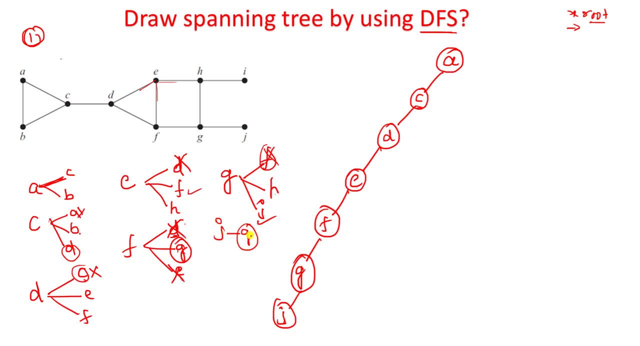 only one vector, one incident vertex, that is g. g is already visited. now we, we are struck here, right, there is no other incident vertex. what we will do? right, we back tracking to the g. okay, come back to g. okay, come back to g. okay, from g again. you see. 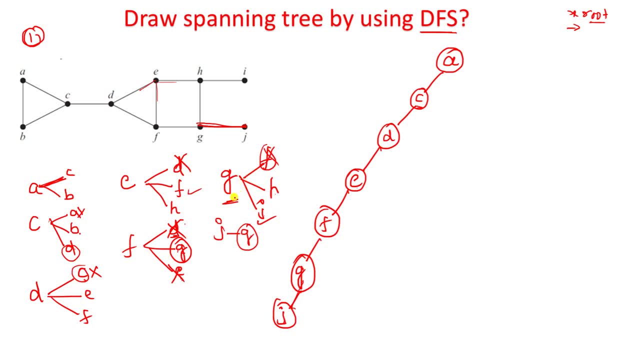 So already, you wrote it right, we already wrote it right. what is there in G, F, H, I. so F is already visited, okay, and from this particular point of view, J is also visited, okay. what is the remaining thing? only H is there. right now, where we are. we are at Z. right, we are at Z. 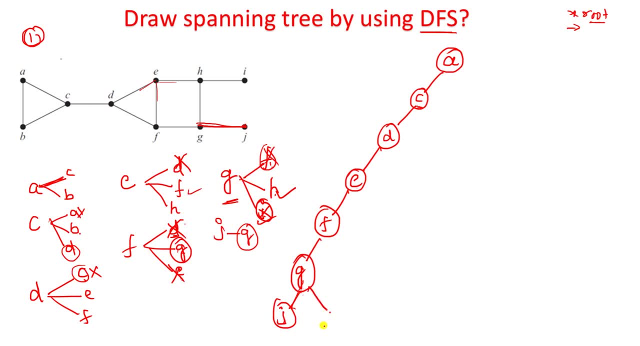 So G have a another incident vertex is what H. Now check whether H- this is our new vertex, H existing any incident one. yes, H have E and I. you see I is already visited and I I not visited, right, so only one element so you can insert here. for H, you have to insert this part, okay, left part of I. 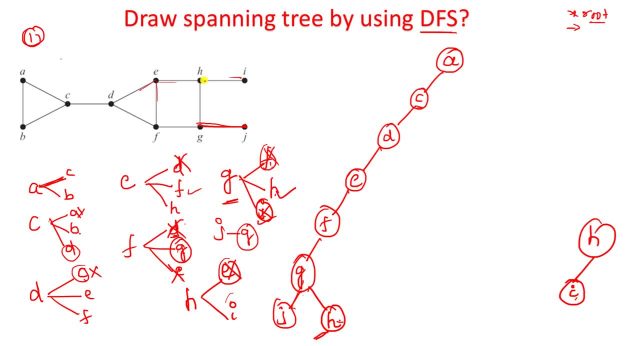 And now again, I, I have only So only one incident: H and H is already visited, so we want to write it again. so this is the stop. we have to stop here. okay, So next go back to H, backtracking, go back to H and come to the H, E and I is completed. okay, go back to G. okay, next visiting. so now G, F, H, I, H is also completed. so what, where we have to go backtracking to F? 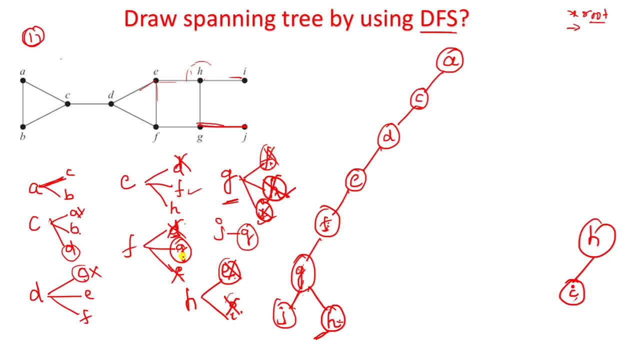 Now check F. F is having D, G, F, F is having how many incidents, D, E and G. D, F already visited and in this case, G also visited. okay, and again go backtracking. and what is the next element? E. so here, in this case, E having F, H, D, right? so all these vertices are here. F also visited and H also already visited. so again go backtracking, okay, D. 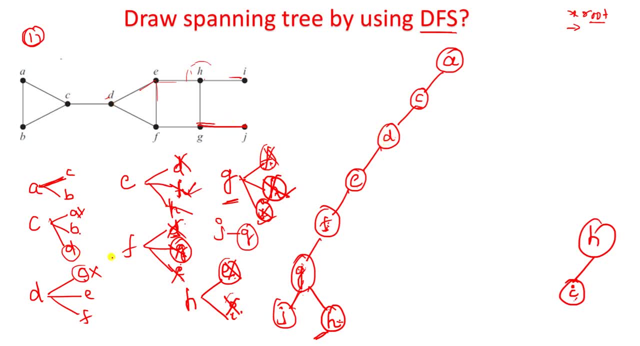 So D is having only one, D having C and E and F3, right? C already visited, E already visited and F also visited. okay, now you are here, now go backtracking. so what is the next element? C? 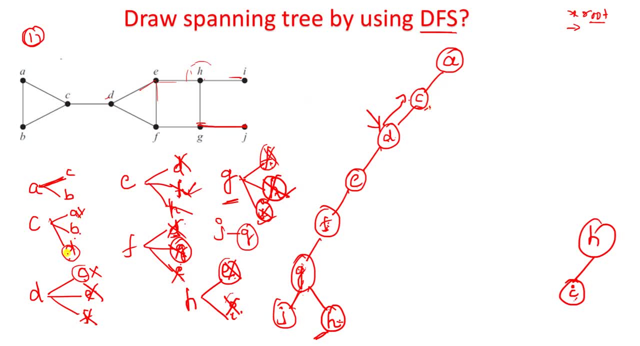 Now C. here C having how many elements? A, B, D, A visited, D visited, but B is visited, no B is still pending. so now here you insert B as a right child of C. Now what is the new element here? 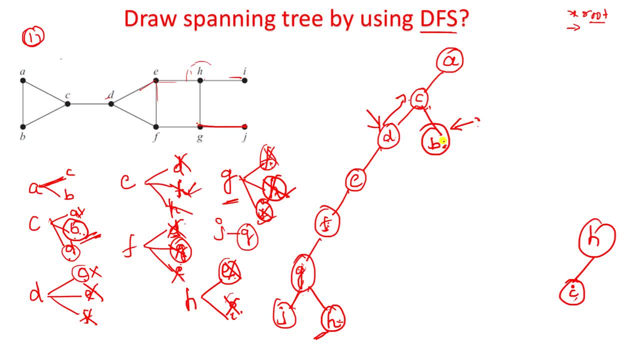 Here B is, Here B is the new element. explore this B. so any other adjacent vertices for this B, particular B. yes, B have a connection with A and C, but these two are already visited right, so no need to take the A and C because A already is there and C also there. that's it okay. 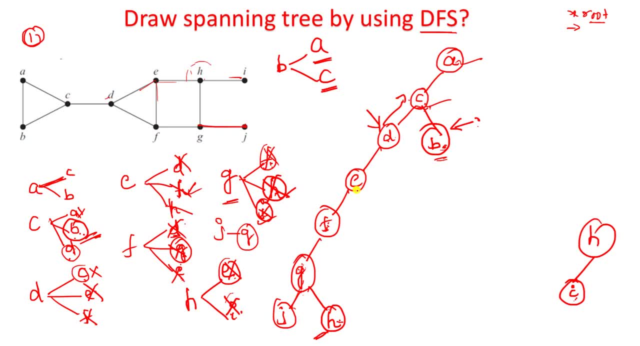 So check it whether all the vertices is visited or not. A visited, B visited, C visited, D, E, F, G, Okay, H, I high here, right, I also visited, okay, so all the vertices are visited or not. so in our spanning tree, in our spanning tree, all the vertices is there or not? yes, all the vertices is there, that's it. 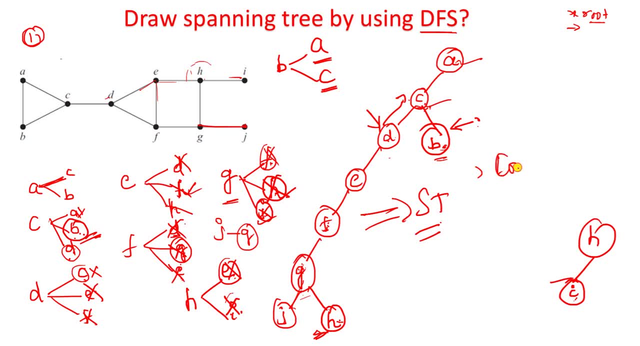 Now check whether this particular spanning tree is a correct or not correct one or not, how we can check how many vertices are there. n is equal to 10 vertices are there, I think 1,, 2,, 3,, 4,, 5,, 6,, 7,, 8,, 9, 10 vertices are there. 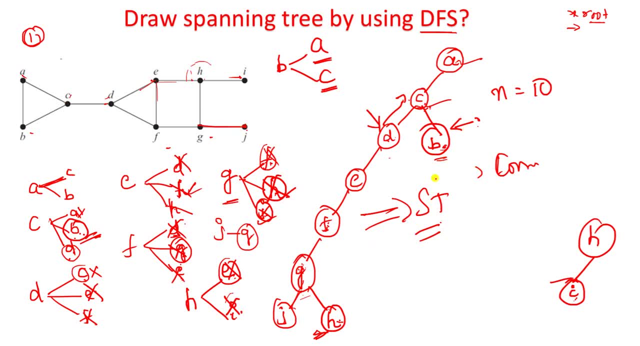 So So our outcome is what, here in this spanning tree, how many edges would be there? it will be there. how many- 10 minus 1, right 9 edges should be there in the spanning tree. so check it: 9 edges are there or not? 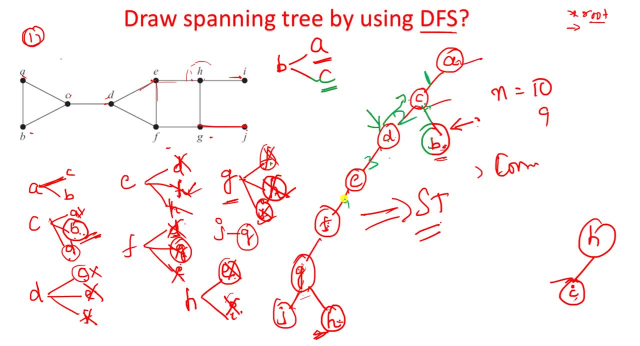 So this is 1 and this is 2, and this is 3,, 4,, 5,, 6,, 7, and this one is 8 and this one is 9, so how many edges? 9 edges are there? okay, so our spanning tree is correct. one, okay. 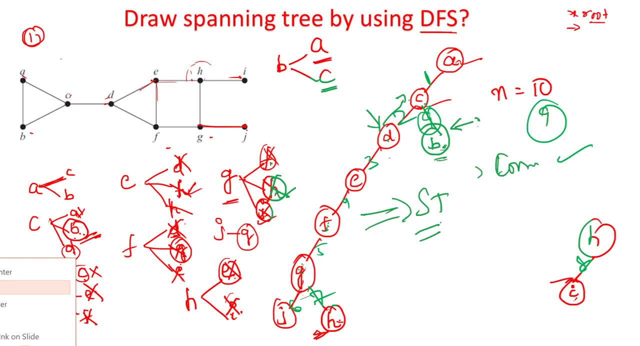 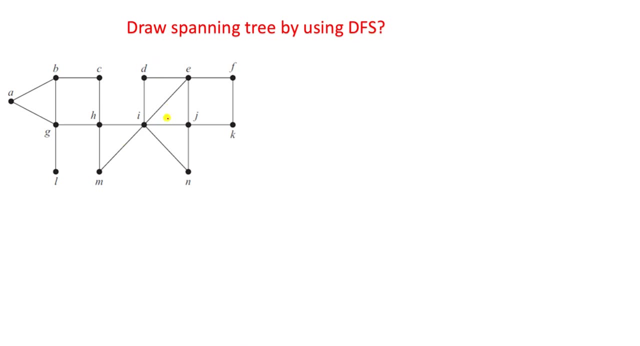 So, like this, you have to do the, You have to construct the spanning trees with the help of DFS. okay, Now we will see another example. So draw a spanning tree by using DFS. So for this particular example also, he mentioned that A should be the root node. okay, 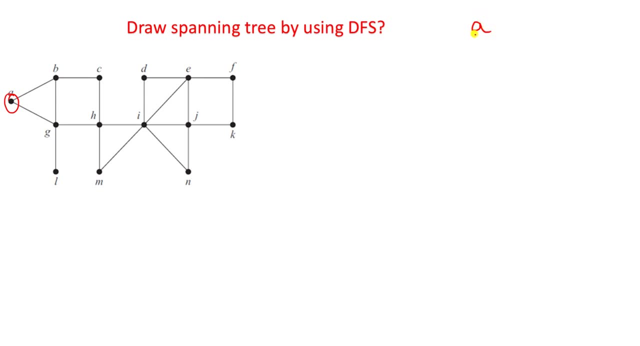 So A should be the root node and what is the conditions? explore this particular vertex, How we can explore. We have to take only one Next Incident vertex. So A have the incident with B and A incident with G. okay, 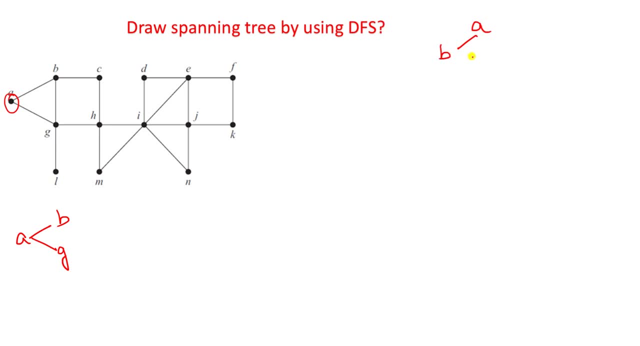 So what we will take, We will take anyone. okay, I will take A to B. okay, So what is the now vertex? is B? Explore B, okay, Explore B. So how we can explore, Write down what are the incident for B. 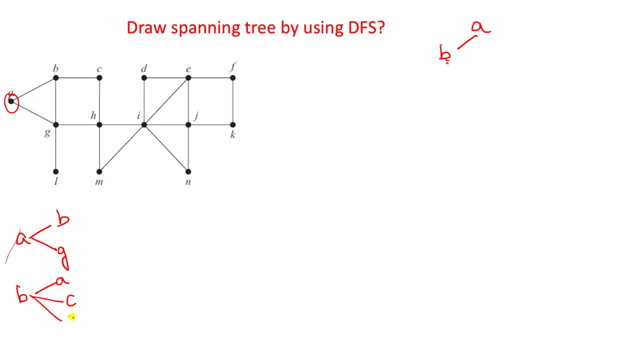 B have the incident with A, B have the incident with C and B have the incident with G. okay, Three numbers are there: B, A, C, G. okay, So I will take G okay, because A is completed, okay. 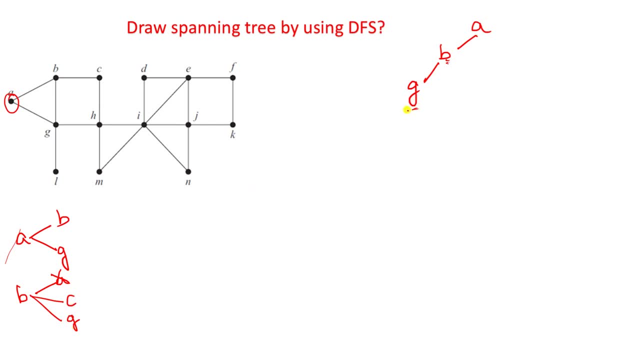 Among C and G, I can take G. So what is the next element? G- okay, G will be the next element. You can take anyone, C or G, any, any of these coach mirror, okay, So this is our new element. 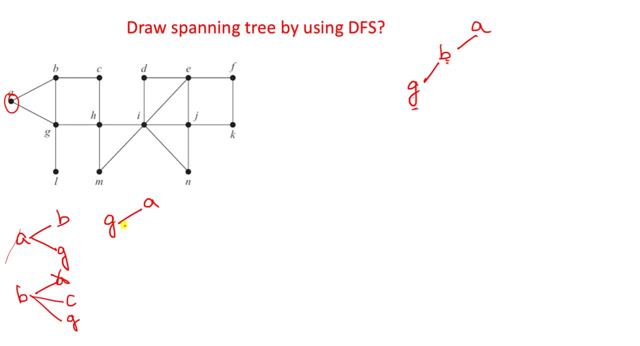 So G, having connection with A, and G, have a incident with L and B and H. Four are there, okay? Well now, So C? A is already visited. and what about B? B already visited, and the remaining elements are what? 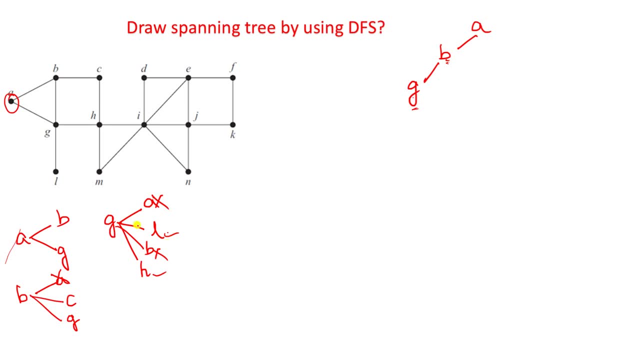 L and H. So among L and H, which element you can take? You can take anyone. So you can take L, L or H. We will take L. okay, So now our vertex will be L. Explore this L. 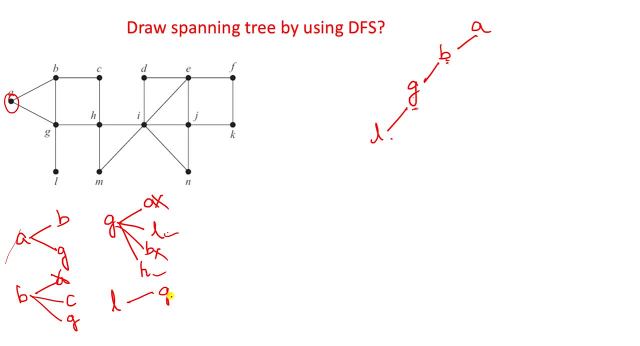 L having the G only one H L having the G only one H Clear, Clear ma. So G already visited, Right, We should not take it again So backtracking. So here in this particular strap, backtracking is started. 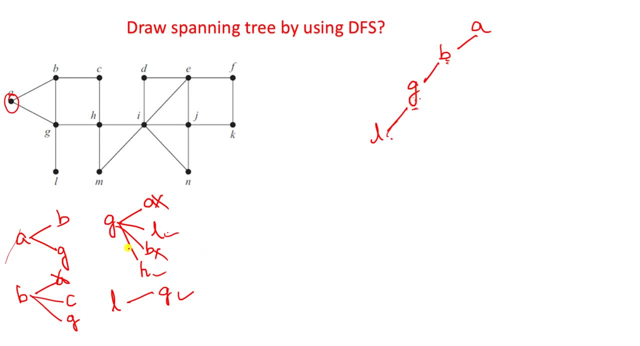 So we have to go back to J. So check it, J, Check it. A is completed, L is also already visited, B is visited, And what is the remaining H? So you have to insert H here. Now, what is the new element here? 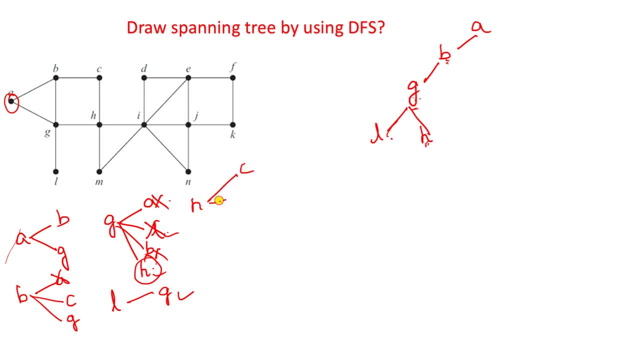 H. Now explore H. H have incident with C, G, I and M. Okay, C, Z, I, M. Is it 4?? Yes, 4 is there? So C already visited? No, no. 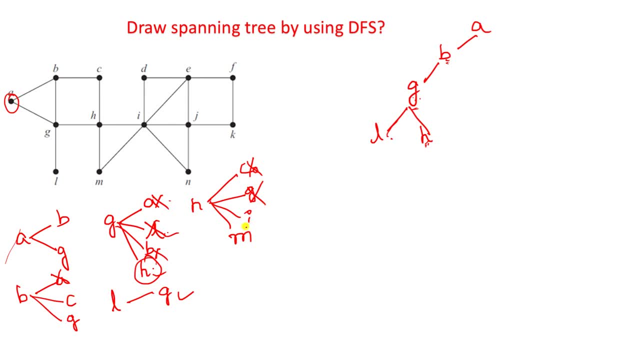 C, not C. G, G already visited? Okay, Is it visited I and M? No, So can we take any one. Yes, you can take M. Okay, Let's take M, So insert M here. 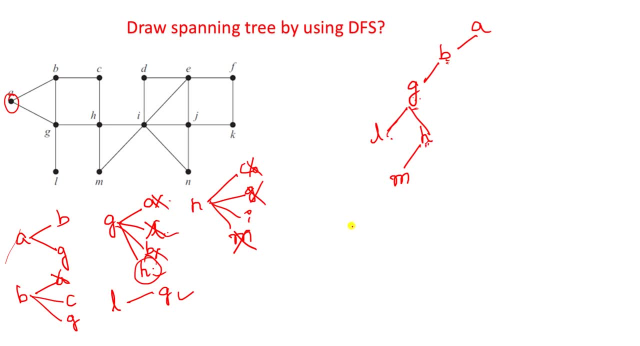 We will take: M So M is visited. Okay, After visiting, let's cross it so that you can understand easily. Okay, ma So M Is completed. Now check whether now our new vertex is M So M. having the edges with the incident with H and I. and what about D? 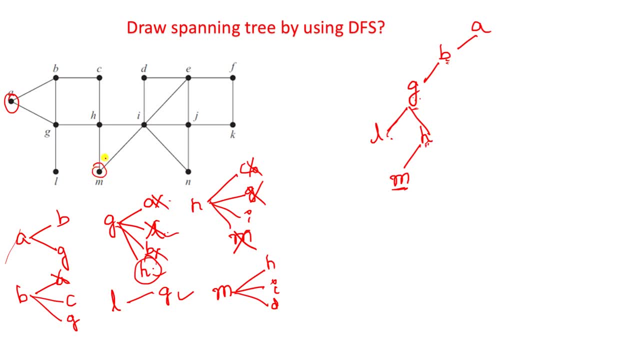 How many? 1, 2.. This is M right. This is M Only 1, 2.. H, I only. Okay, Not D, Only H, and I. So see H is already visited. no. 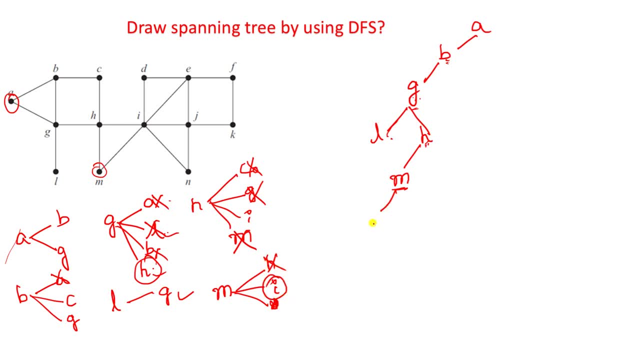 Yes, Right. So what is Now? only element, Only I is the remaining element. Now check, I See here. What about I here? I here. So how many elements are there? 1,, 2,, 3,, 4,, 5,, 6 edges. 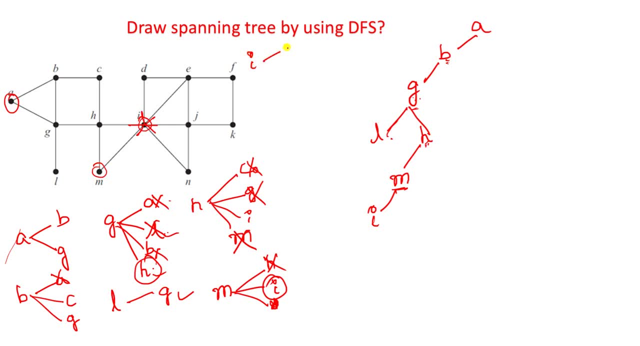 6 incident: vertices are there? What are those For I, H, D, E, J and what is this? N and M Right? M is visited already. H is visited already. D is not visited. E is not visited. 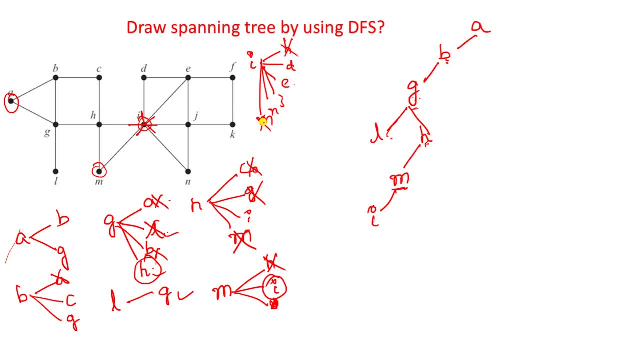 J is not visited, N is not visited. You can take any one of them. Okay, We will take J. Can we take J? Yes, So insert J here. Okay, Now explore J. How we can explore the J. 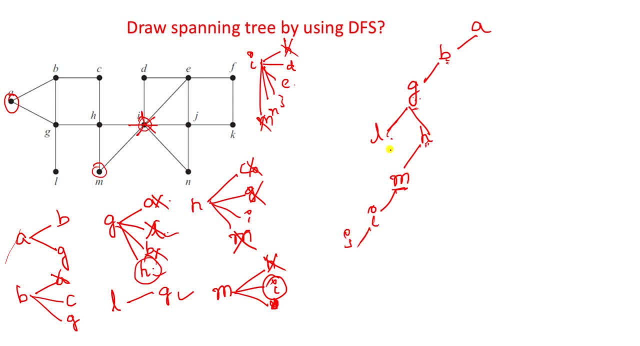 See here J, here, So J having how many vertices: 4 vertices, incident vertices: J having E and K and H. So this is the J Now how many vertices, 4 vertices, So J having how many vertices. 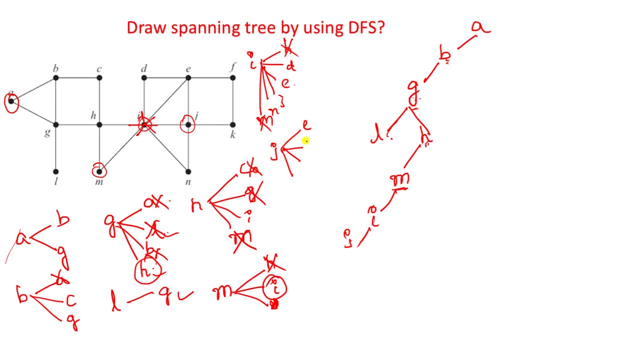 4 vertices- incident vertices J having E and K and I have N and also I. Okay, So among these, I is already visited. What about N? N is not visited, And what about K? Not visited, And what about E? 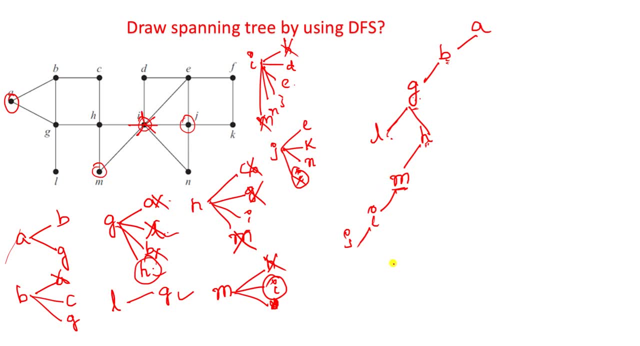 Not visited, So can I insert any one of them? Yes, You can insert E, K, N, So I will take here E, Okay, E, E as a next vertices. So my new vertices is what E? 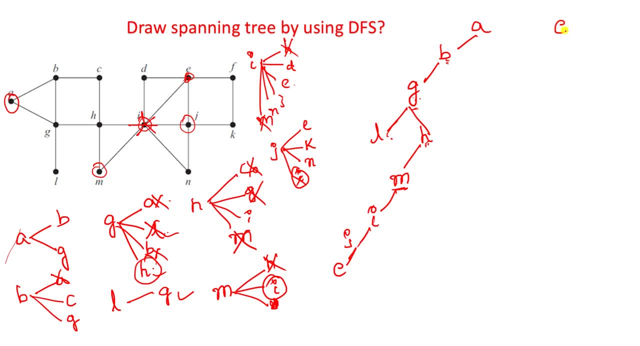 Okay, So check it. What are the adjacent vertices for the E? E having 3, 3, incident D, F, J. You see J is already completed. What about F? F not completed? And what about D? 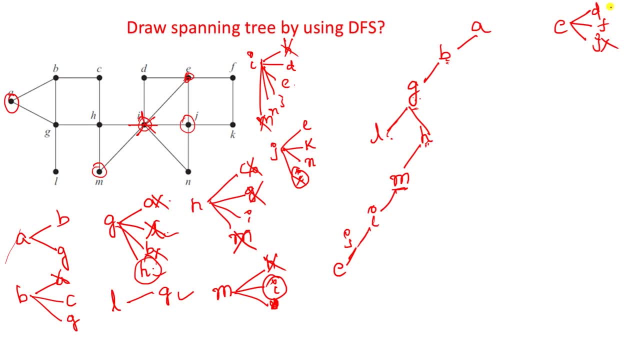 D, also not completed still, Okay, So you can take any one. Yes, I will take F. You can take F, Okay. Or D Any one, Any one. Or you can take D, Okay, I will take D here. 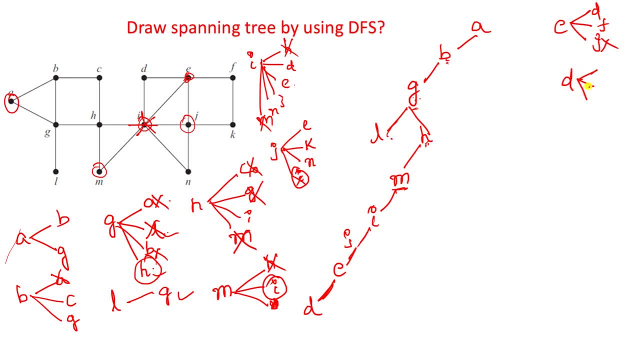 Now check. You can explore the D Now D check the. what are the incident for the D? D having only 2 incidents. That is, D edge with E and D have a path with I. Okay, See here E and I, both are visited. 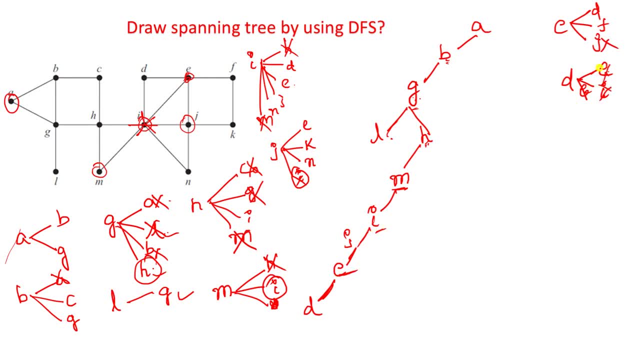 No, Here. E is there, Here, I is there. So both are visited, So no need to write it again. You should stop here. So stop here and go back to backtracking E Now. check E here. Where is the E? 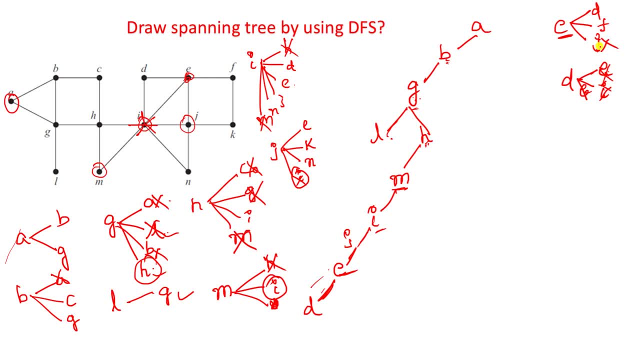 Here. So what is the path existing? J already visited, D already visited And what is the remaining element F? Now you have to insert F Now check F here. Your new element is what F Now F will be. F is having, K is a one path incident and F is having a path. 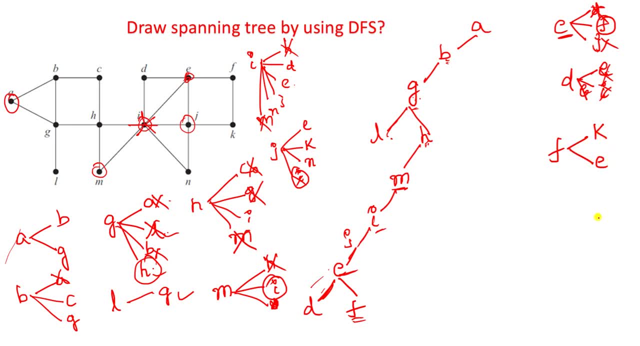 Okay, F is a path with E. Okay, F, E and F, K. Now see here: E already visited Right, So you can eliminate this one. And what is the remaining element only left with here K, Right. So for F, we have to insert here K And explore K, Explore K, So K having what is the element? 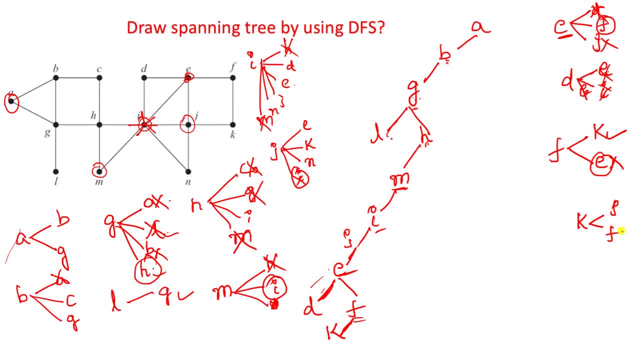 J and F. J and F. You see J already visited, F is already visited. Okay, So there is no other elements. incident with K. So we should stop here and we come back. Backtracking has to be done. 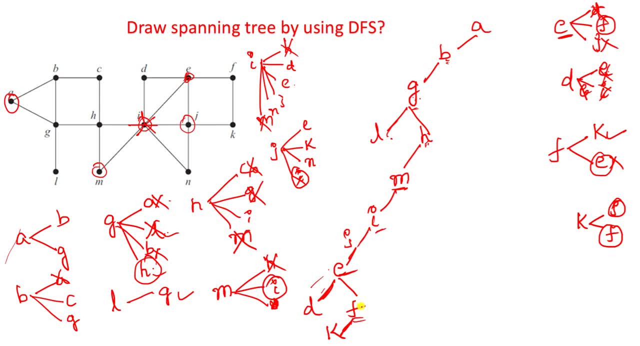 So we come back to F and check with F, F having only two incident, K and E. Those two are also completed- And go back to E and check with the E. E is having three incidents: D, F, G. Those three. 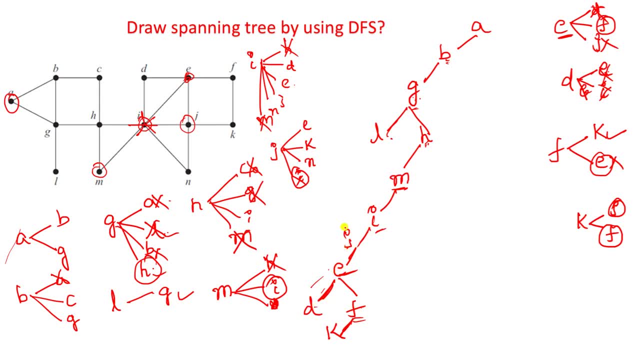 are also completed. D, F, G also completed. So you can take, you can go back to J and check with J And here see this J here. So E is completed. K is completed, Am I correct? 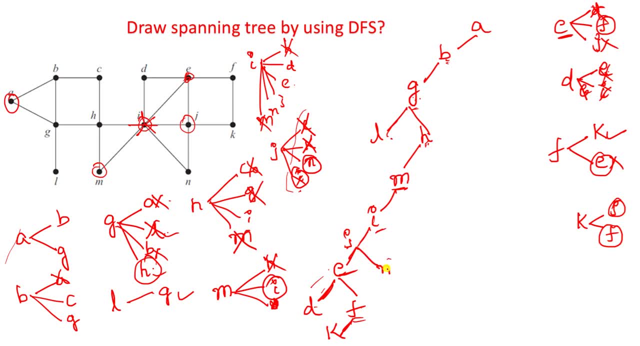 So what is the left with here in J? Only N. Okay, N is there. Now what is your new vertex? N? Check with N. Okay, Write it down here. N, N is having how many vertices? two vertices, incident with the J and I. You see, I and 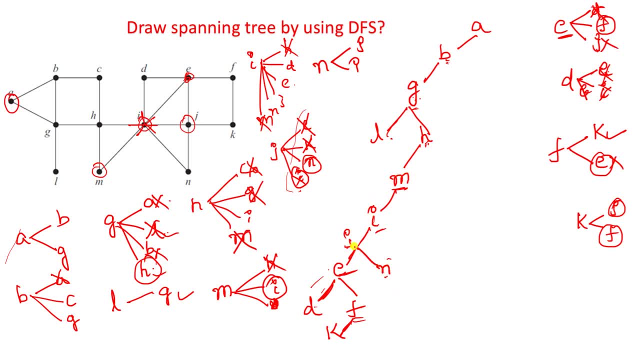 J already visited, So no need to write it again. So go backtrack to J, backtrack to J and J: all the vertices is completed. all the vertices is completed. and come back to I and check with I at I: D is completed. no S D completed. what about E? E completed. what about J? 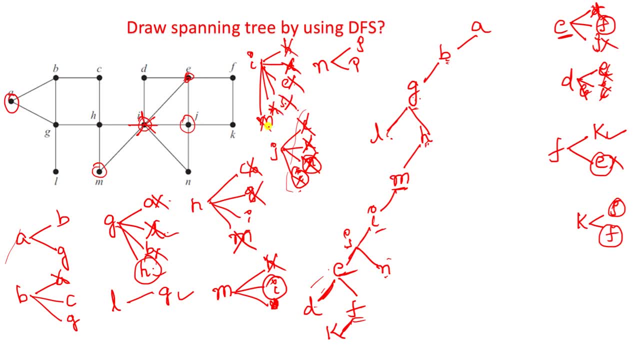 completed. what about N completed? and what is the last one? M right, so I is having D E. H is completed, M completed, N completed, J come. all the elements are completed, all the vertices we visited already. so come back to m now check with m m, having only left with i, but i already visited no. 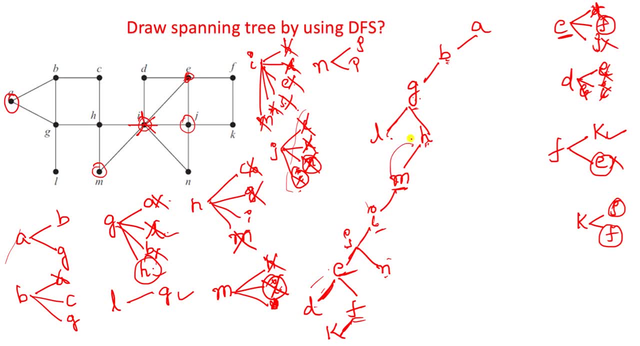 so you can eliminate this one. so go back to h. so check with h, h having c z. i m right, so i already visited, so you can delete this one. so from here you can go go back to or backtracking to g, right, so at the z we have h, a, l, b, h. so see h is already completed, ma this also visited, so no other. 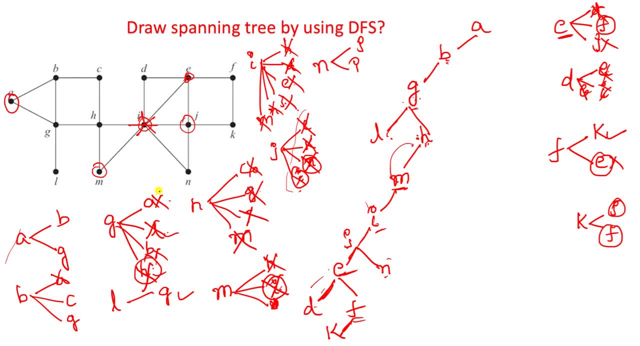 elements. i think g having l also right, g having, yes, l is also completed. l to g: l is also completed. okay, so g is having a, a completed and h is completed and l is completed and b is completed, and now go back to g. so, and now go back to b. so b is having only one incident, that is, a and a only visited. so no, 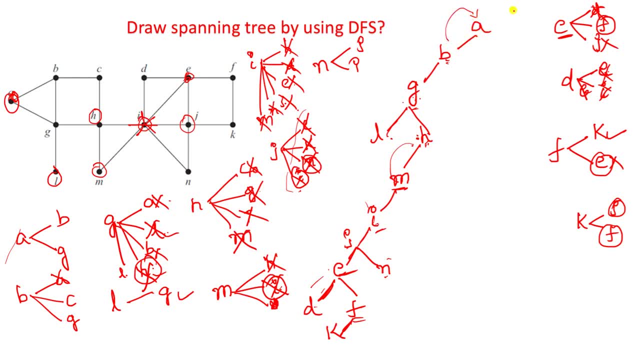 need to write again. and finally we we come back to our root node b. okay, so still any element spending with root node b and g. only two incidents for the root node b and g: b visited, g visited. so all the, all the root nodes, all the vertices, what are there in the graph is visited, ma. 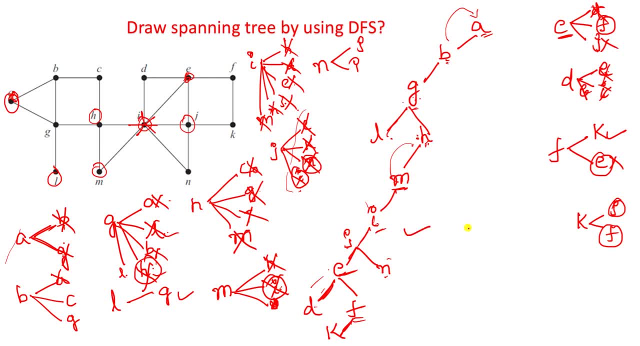 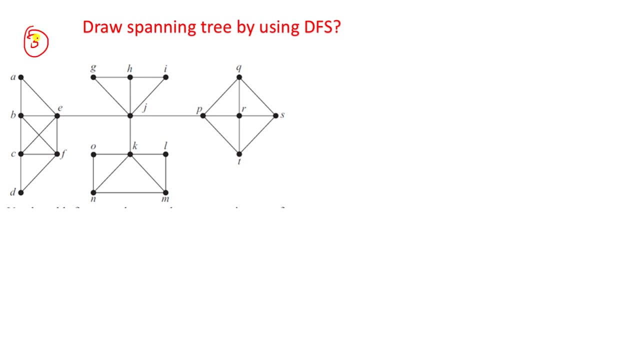 this is also fifth iteration, this vertex, and then explore it. explore it to what is the first vertex: incident. ok, you can take anyone among them among the incident vertices. so a having connection with b for this particular graph b and e. ok, first check how many vertices: 1, 2, 3, 4, 5, 6, 7, 8, 9, 10, 11, 12, 13, 14, 15, 16, 17. 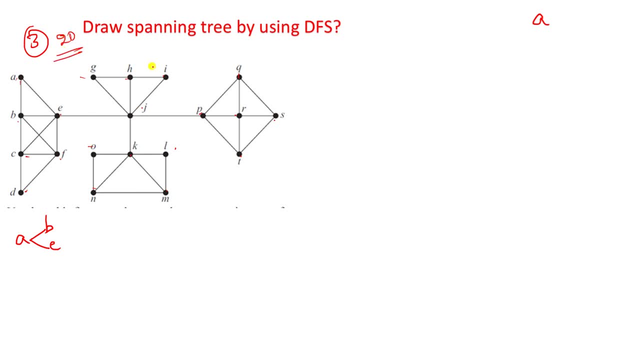 18, 19, 20, so almost 20 vertices are there, so we will get almost 19 edges will be there. ok, in our particular spanning tree we will get almost 19, not more than 19. ok, if you get more than 19, it is not the spanning tree you can. 19 edges are not the spanning tree which. 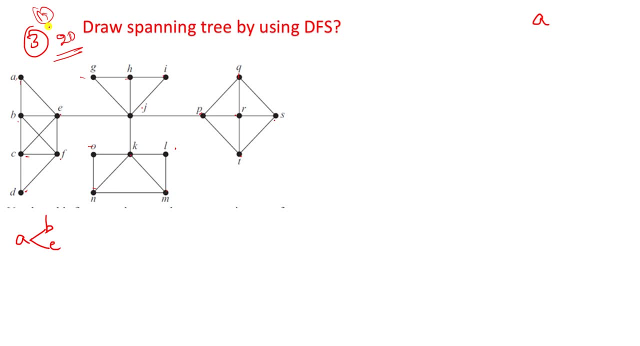 is wrong. check it: 19 and 19 should be less than the spanning tree. ok, so here see a have connection with b and e. right, so directly, right. so what we will take. can we take b? ok, b here, and the next one, b, is completed so you can eliminate this one. and what is the next? new vertices b and explore. 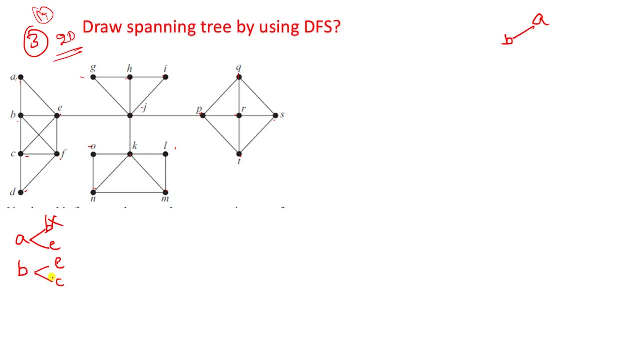 b, b having e and c, and also a. a is already visited, only to write again- and f- right, so three elements are there. b having connection with e, c, f. right, so we will take e. can we take e? yes, you can take any one, ok. e, c, f, so check with e. e having. 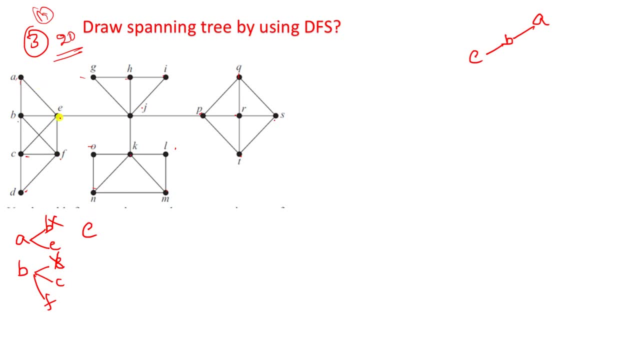 incident with a and b, a, b, a, b already visited. so what is the remaining one, j and f, j and f? ok, so can we take f. i will take here f. ok, so f is visited. so where is the remaining one, j and f? in between, e and f is the same right and where is where is the f? where is the f here? due s Their business. 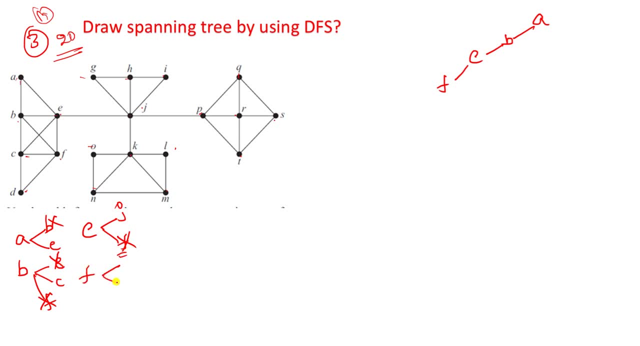 and here it says that visited. ok, now what is your new? where takes f? so right, and what are the vertices? b, be of business, only try it again. e, e, Videntified and see, see, not listed, so I don't see. and remaining one are d. so among the C and D you can take anyone, so I take here c. ok, so C is visited, right out. and 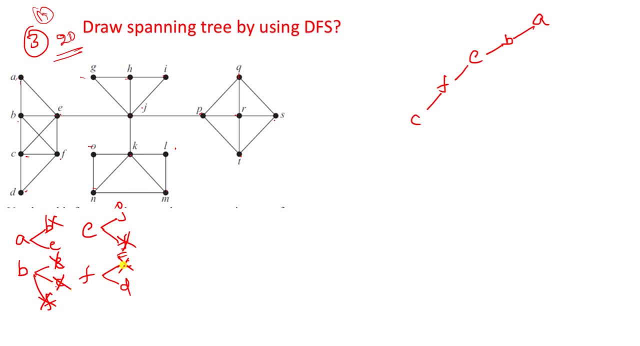 here below cut. thank you, I want To seeан body, this The visitor. no, so You can eliminate this one or write d on here and this. So you Now. what is the next element C? right, What is the next element C, not D, Don't be confused. So, C explore, C, C explore 2.. C have incident with B F D, B F D, But B already visited, F already visited and it remaining, you see, C having actually B E, F, 4 incidents unna hai mani ki. 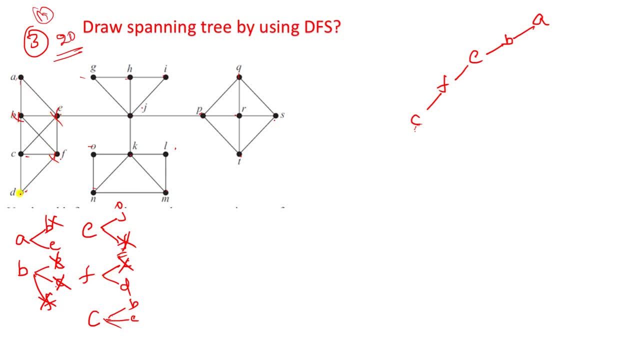 Ok na, But B completed, E completed, F completed. So only one element is what D? So you can insert D here. Ok, You can take it any order, ma It is not mandatory to take F first or C first or D first. Ok na, Among those elements, you can take any one. 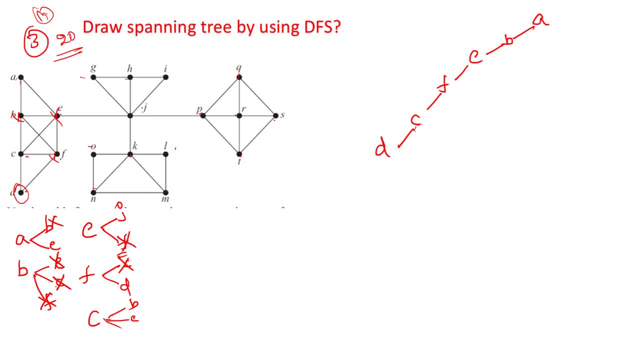 Kabatty andhra ki okokali ki okola ussundi Graph annati, For example, ikka nino B degri E teeskundanu E kaakonda mir C teeskundar ankondi. It will be change, right. And what is my next element D? Now write down what are the incident vectors for the D? So D having C and F, C and F only. So C, F and A already visited, right. So we should stop here. 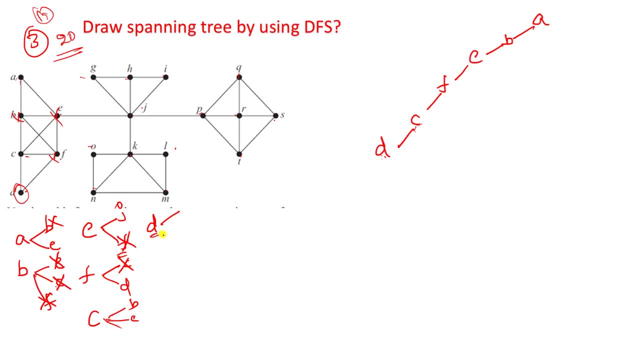 Because there is no other elements for the D. So what we have to do, We have to backtracking right. So from here we have to move: C Now check C, Check with C. Check visited B, F, D, E also. 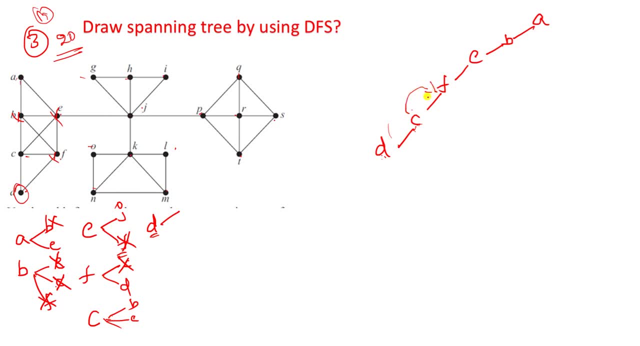 So there is nothing like that. other elements with the c. so again backtracking to f. okay, from here to here, and from here to here, we are moving. and next one, f check with f. f is having d d already visited. no, let's see. so 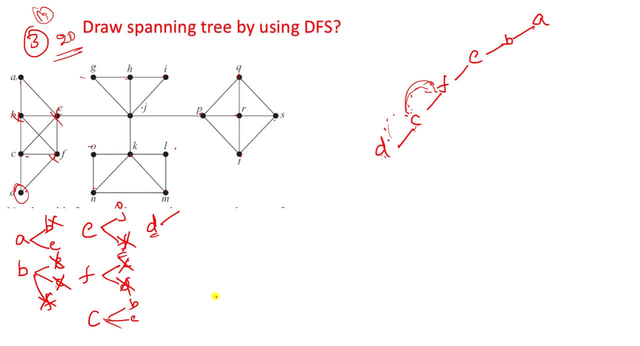 you can eliminate this one right, b and d. so d completed, b completed right. so f is also visited. so from f to we have to move backtracking to e. so check with e, f, j, so still j is pending, so you can write j here now what is our new element j, and write down what are the incident vectors. 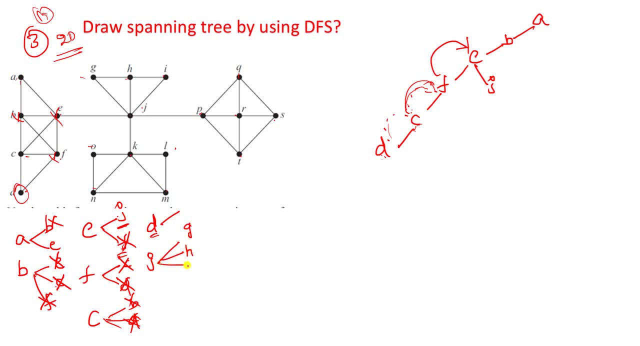 for the j. j have connection with g, h, i and also e. so e already visited, so let me write it again. and p and k. okay, you see one, two, three, four, five, six, but this one is already visited, so we have to move backtracking to e. so check with e, f, j. so still, j is pending, so you can. 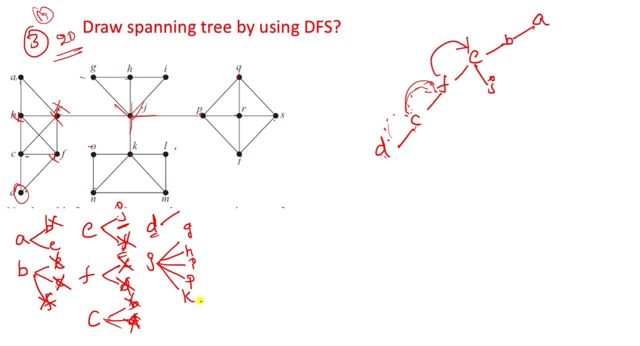 write j here, so 5, 1, 2, 3, 4, 5, so among these, anyone visited? no one is visited, so you can take anyone. so can i take g? yes, you can take g here, okay, so among these you can take anyone- g or h or i or p. 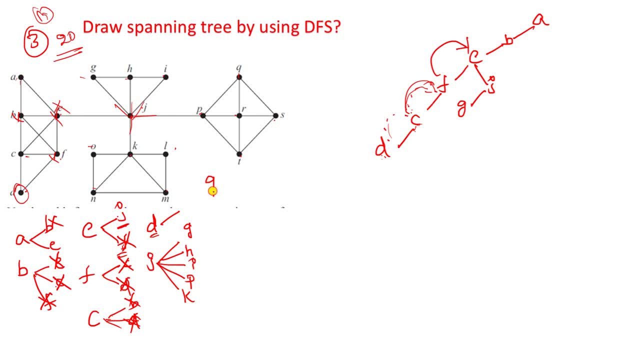 or k. okay, g is our new vertices. now write down what is the next vertices, next incident vertices for the g. j has having only two vertices, h and i. i already visited, so we have to move backtracking to e now. what is our new element? j, and write down. 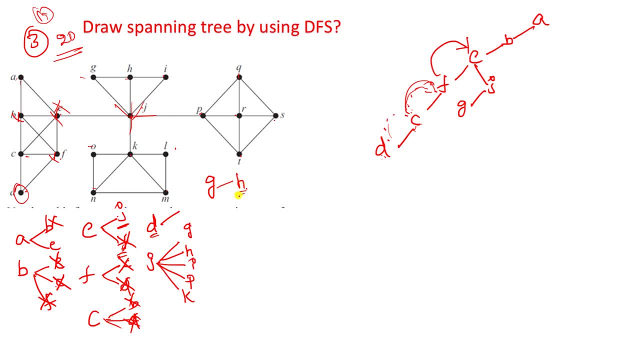 visited. so g is having only h, so stay, h is visited. no, so i can insert h as a next next vertices. okay, next, what is our mu vertex h and explore this h. h is having two vertices: g and i. g already visited and the next one, i. actually, this is having three, but these two are already visited. so what is? 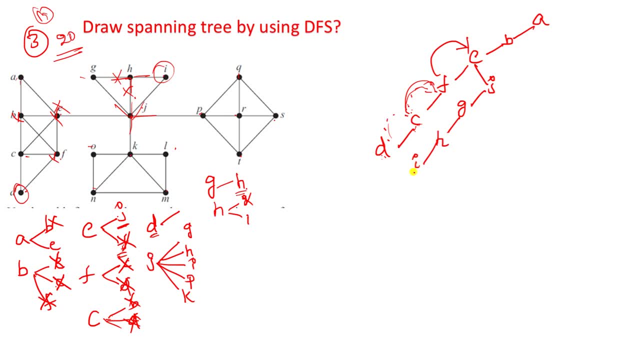 the remaining element i, so you have to insert the i. okay, and what is our new vertex? i and come to the i and explore it. so does i existing anyone i having i? actually i having h and j, but these two are already visited. so from this point you stop here and go backtracking. and h still still any. 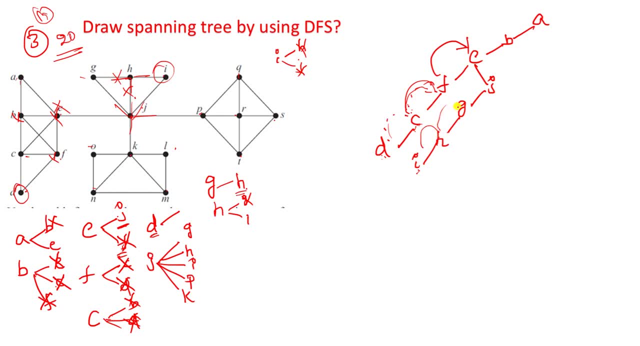 elements: vertices is pending in the h, no, so go back to g. so still any pending no. all are completed. incident vertices: all are completed. the g, so backtracking to j. so see here. right, so so, and j. g is completed, right, h is completed, i is completed. and what is the remaining two elements? 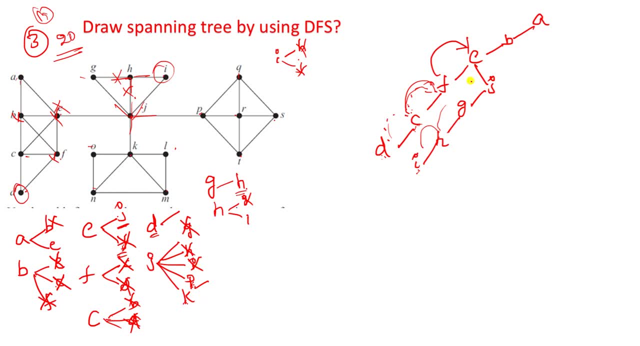 p and k. okay, take any one. I will take p. okay, I will take what p Now explore p, explore p. so what is the elements? p q, p have incident with r and p incident with. 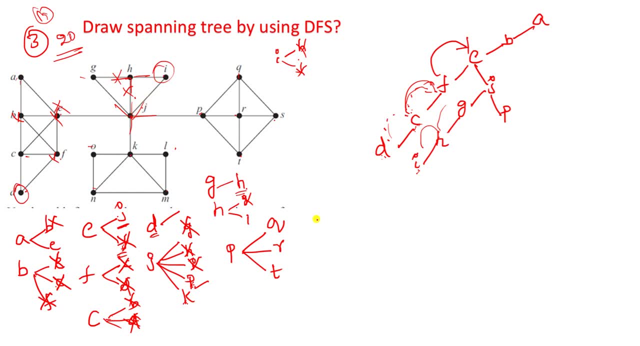 t p actually incident with j. j already visited so I do not want to waste the place, so I am not writing the already visited vertices. okay, hope you understand. so q or t. among q or t, will take any one. I will take q, okay, so q visited. now explore q. q having p. 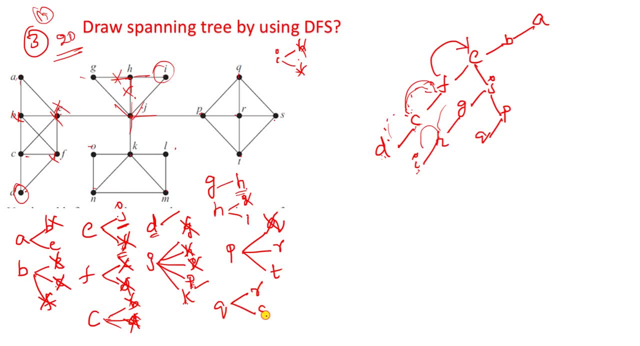 p already visited q having r incident and q incident with s. so among r and s, among r and s will take any one. I will take r. okay, I will take r. so r is visited ma here p also, we have the r, so you can. 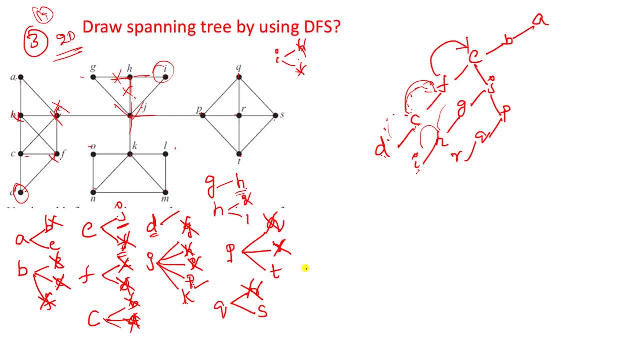 visited this one, so eliminate this one. and next, what is our new vertex? r right, our new vertex is what r? so explore r? r having the q q already visited and r have r incident with p visited and the remaining two s and t? s and what t s is visited? no, is t is visited. no, you can. 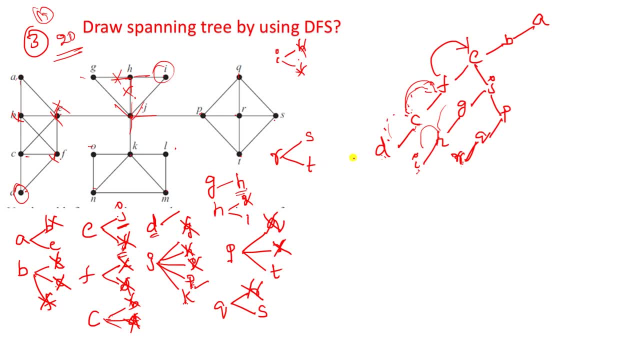 take any one. Can we take q, s or t? we will take s. okay, we will take s. so s is removed from here and s should be removed from here now. check s where we are. s right s having incident with q and r entity. 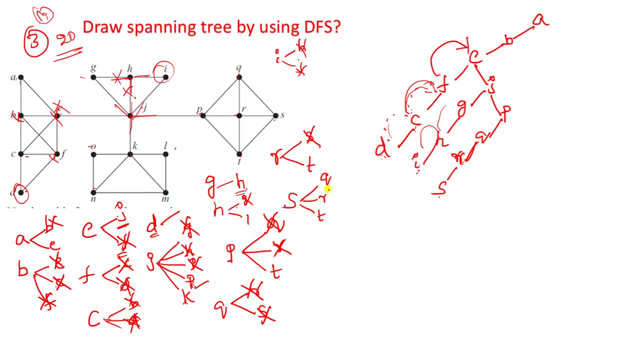 yes, incident with q, r and t. but q is already visited, r visited, and what is the remaining element? Only t. okay, so t anywhere here. yes, for this particular p also, t is there, so you can eliminate. 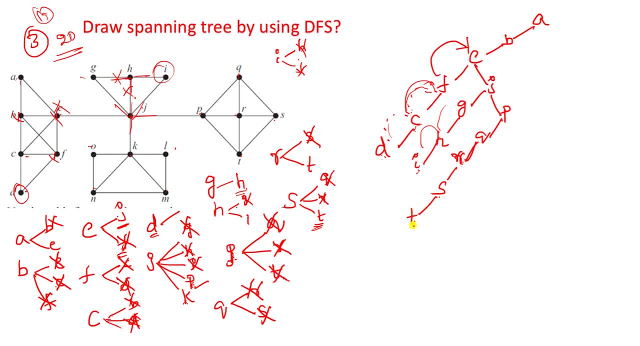 this one. so now the next element will be t. so t is having any incident. yes, t have incident with p and r and s, but these all three are already visited. p is there, r is there and s is there. right, so now how we can do, we have to backtrack into the next. 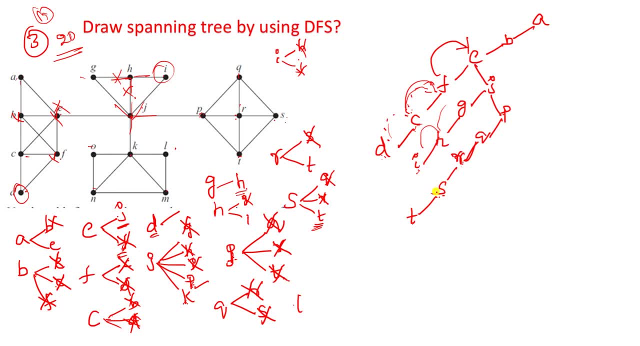 part s. so from here s to, we have to move. is there any still pending? r is completed right, so from s to we backtracking to r. so at r any still pending r is t is all completed so. 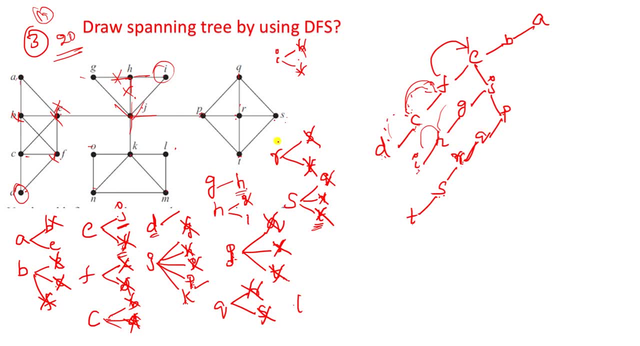 from r to we backtracking to q, so check it q. q having only two now: p and s, so p and s. both are visited, so we backtracking to p, so p is having j. all these elements are completed. 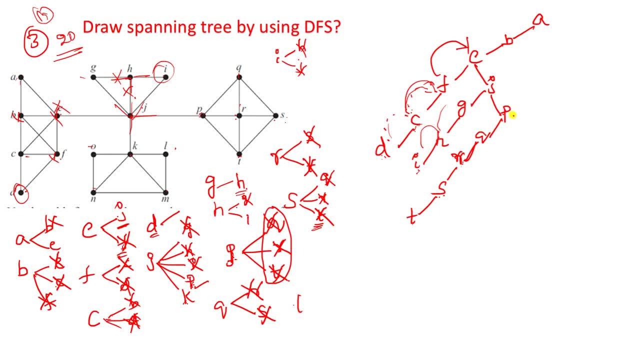 right at p. all these elements are completed. so again, backtracking to j. so from j, any vertices is still pending. yes, k is pending. what is that? k is pending, so can we insert the k? yes, we have to insert the k. okay, explore k now. explore k now. so. 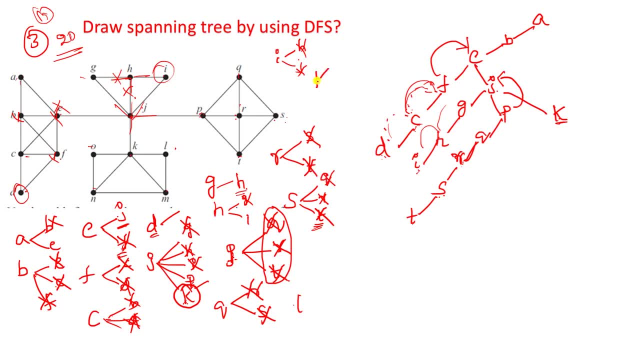 so what are the next incident vertices for the k ma k having o. j is there, but you can eliminate that one. j already visited. so k, l and n and m. four vertices have right. so can we take any one? yes, you can take o. you can take any one o all n m low. 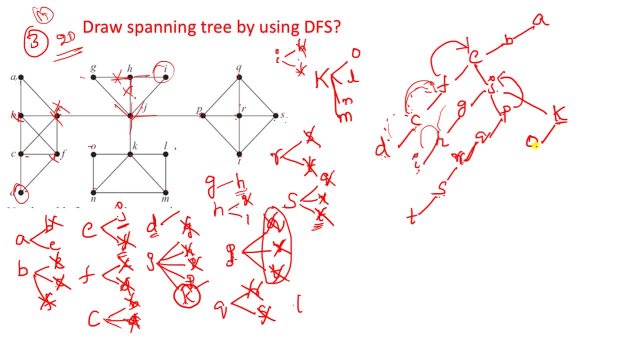 algorithm with this code. so i will take here o and my new vertex is o and i explore backtracking to j. now explore k. now explore k. now explore k. now explore this vertices. so now check o having any new vertices. it is incident with k and n, but k. 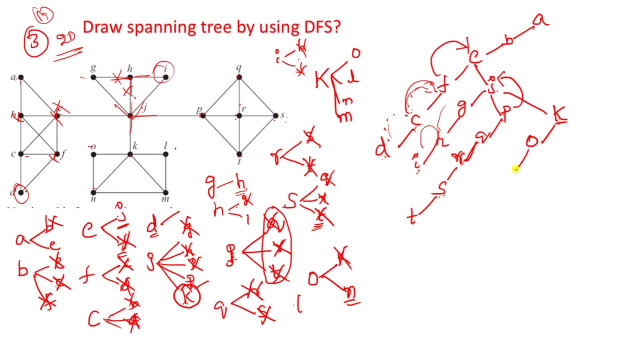 already visited, no, so no need to take. so what is the left element? only n, so you should take n only and you explore the n. n is having two vertices again. okay now, o, k and m. o already visited, k already visited. and what is the remaining element, m? okay now, our new vertices is m. 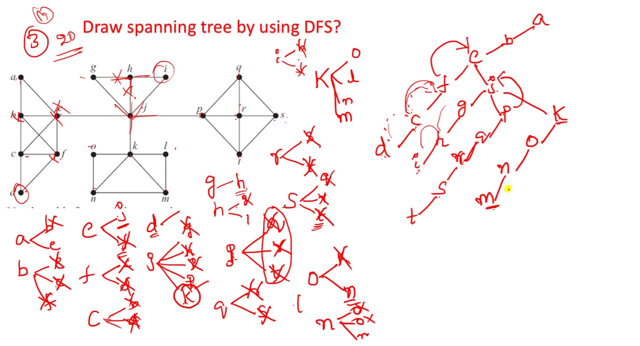 right. my new vertices is what one. m explore this m how we can get m having how many vertices. m incident with k. m incident with l. m incident with n, but here still n is completed and k is completed. what is the remaining element, l? l should be inserted here and my new vertices will be l. 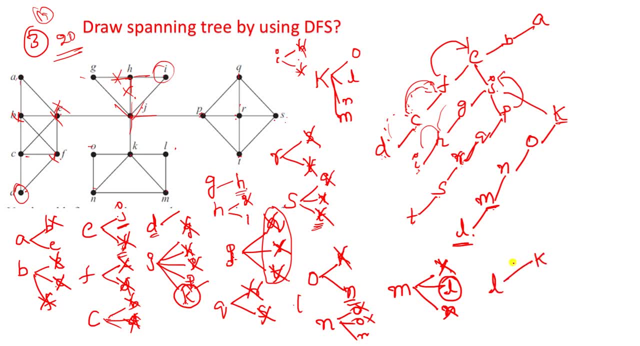 okay, explore the l. l have a connection with k and next to any anymore elements, l have a connection with m. okay, so k already visited. no, no need to take. and m is also visited- no need to take. and here we stop the session and just go back to m. still any, any. 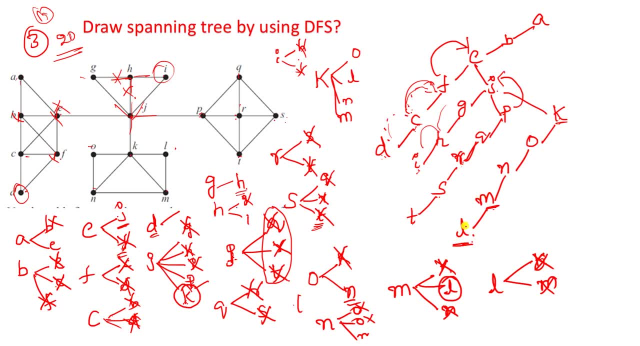 we should not stop like this. we have to stop here and go back tracking to m. still any more pending in the m? there is no pendings. l is visited, okay. and go back to the n- there is no pendings. and go back to the o- there is no pending. and go back to the k- there is no pending. is there any elements here still? 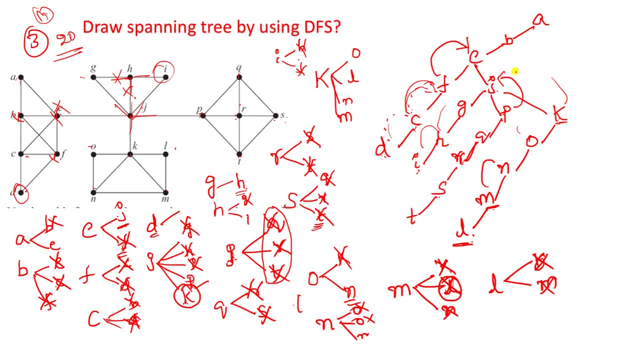 pending with k. no, there is no pending right and go back to j and go back to e and go back to b and finally go back to a. okay, so there is no elements are pending until you reach all the elements. so still: 1, 2, 3, 4, 5, 6, 7, 8, 9, 10, 11, 12, 13, 14, 15, 16, 17, 18, 19, 20 elements are there. 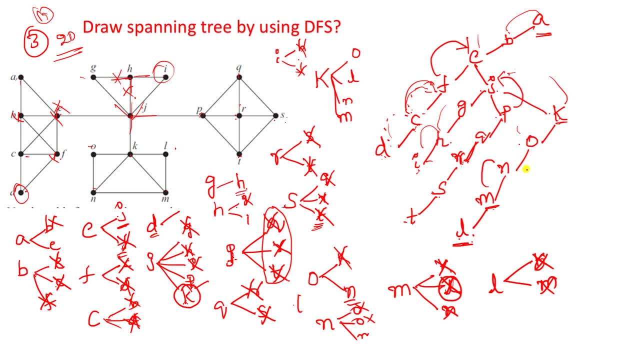 now check how many edges are there in this particular spanning tree. okay, see, this is the one first, and this is the second and the third, fourth, five and six and seven and eight and nine and ten, eleven, twelve, thirteen, fourteen and fifteen, sixteen, seventeen, eighteen, nineteen, see 20 vertices. 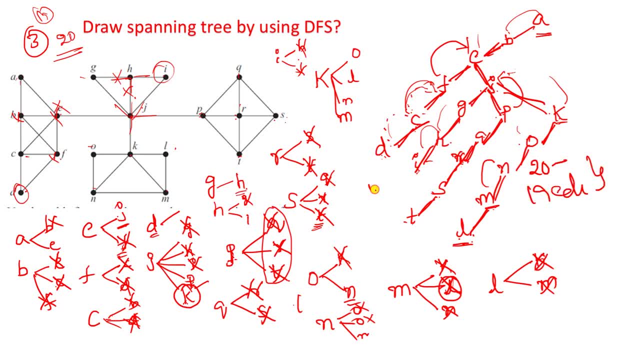 19 edges is the spanning tree. yes, our tree is correct, one right ma. so like this, you can draw any, any spanning tree. okay, here, for example, i took a to b, you can take e. so it is something. a structure will be changed. spanning tree check structure will be changed, but we can construct any number of spanning.